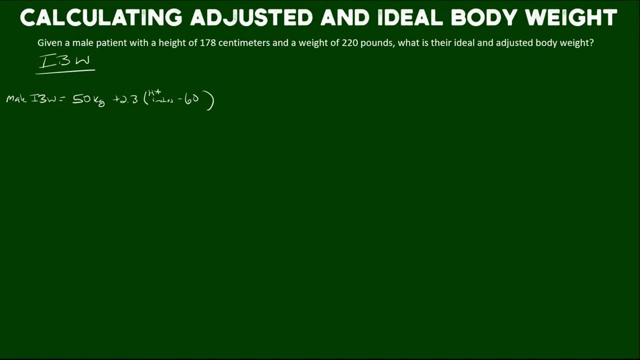 their height in inches minus 60. And I also want to point out that it's a little different for a female, And the only difference being it's 45.5 kilograms plus 2.3. Times height in inches minus 60.. So that's what the equation looks like. So can we do this equation? 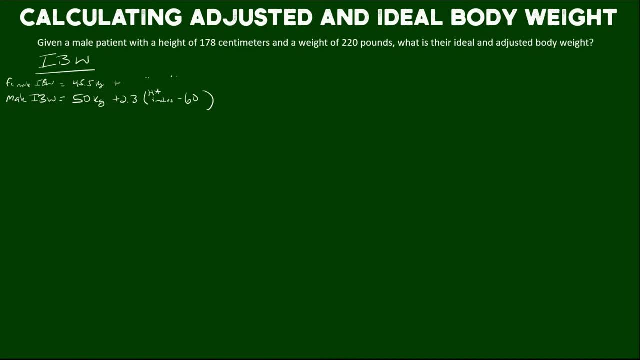 yet, And it doesn't look like we can because we don't have their height in inches. So let's figure out what their height is in inches. For a patient with 178 centimeter height, we would multiply by the conversion factor to turn centimeters into inches, which looks like this: One inch having 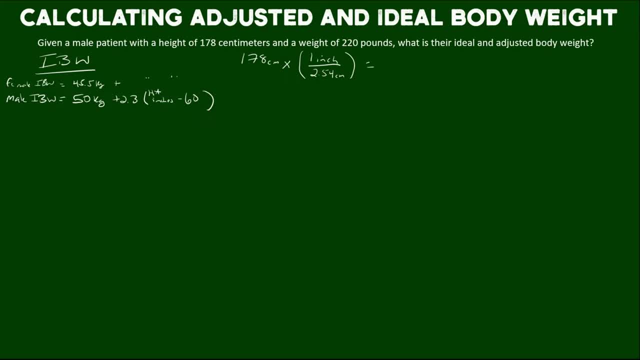 2.54 centimeters in it And if we did that math, this patient's height is about 70 inches. So now that we have that, we can go ahead and calculate their ideal body weight. So this patient's ideal body weight is about 73 kilograms. So let's see what that looks like when. 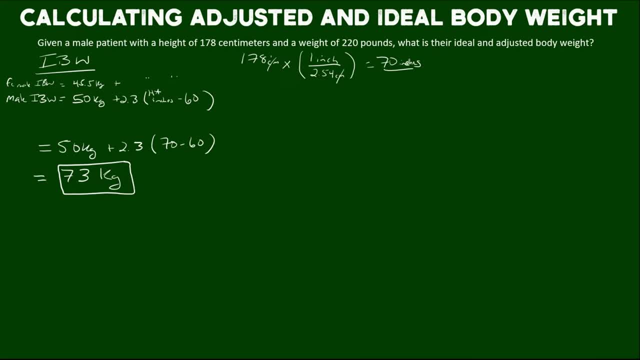 we compare it to their total body weight or their actual body weight of 220 pounds. So let's convert pounds to kilograms. Multiplying by the conversion factor for pounds into kilograms, this patient has a total body weight of 100 kilograms. So you can see they're quite a bit higher than their ideal body. 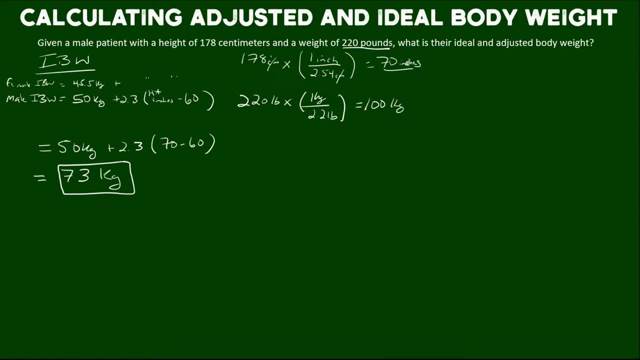 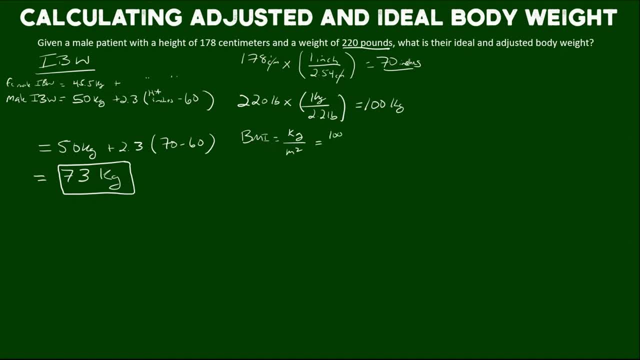 equal to kilograms. So BMI is equal to kilograms. So BMI is equal to kilograms. So we have kilograms And if we multiply the centimeters times 100, that converts centimeters into meters And we need to square it And that gives us a BMI of 31.6 kilograms per meter squared. 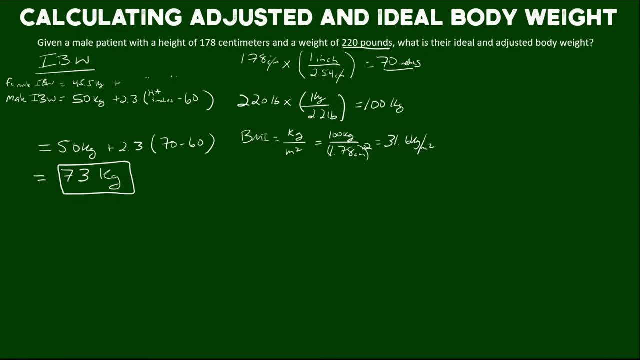 And if we compare that to the charts of BMI, which include 18 to 25, being normal weight, 25 to 30, being overweight and greater than 30 being obese, we can tell this patient has pretty high BMI in the obese range. 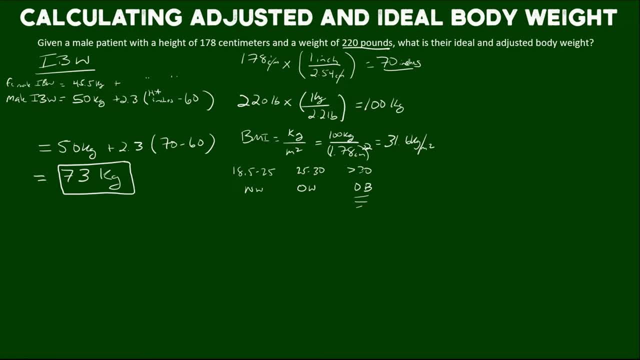 So we've calculated their ideal body weight. Let's look at how to calculate their adjusted body weight, And that's with the following equation: And what adjusted body weight is is what it says it is. It's really an adjustment usually used in certain dosing. 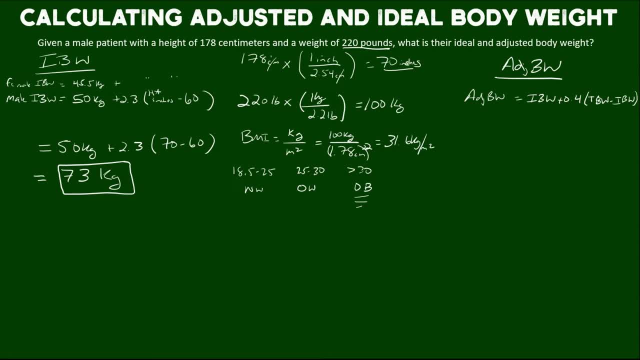 or pharmacokinetic scenarios where a patient has a very high BMI And we need to do some sort of adjustment because they're just nowhere close to the ideal body weight. Therefore, we could be underdosing them or potentially incorrectly calculating something like a renal 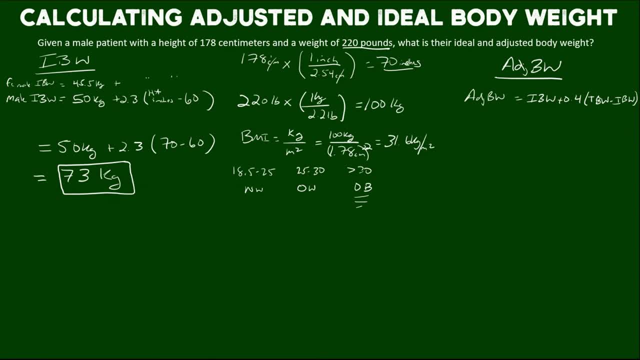 clearance if we don't use an adjusted body weight. So for this patient the calculation of adjusted body weight would be the ideal, plus 0.4 or 40 percent adjustment times 100 minus 100, which would be the total body weight minus. 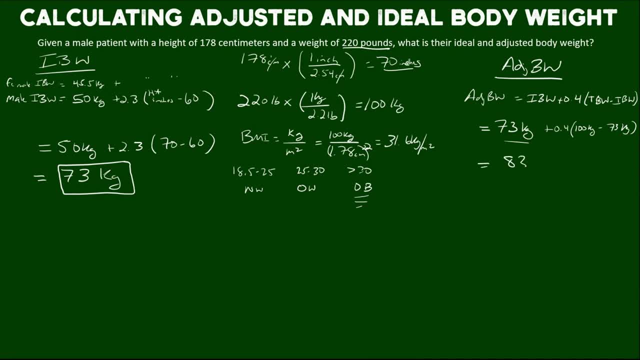 the ideal body weight And that gives us an adjusted body weight of 83.8 kilograms. You can see it lands somewhere in between the ideal body weight and the patient's total body weight of 100 kilograms. So this video just kind of wanted to go over how we do these calculations. Some calculations: 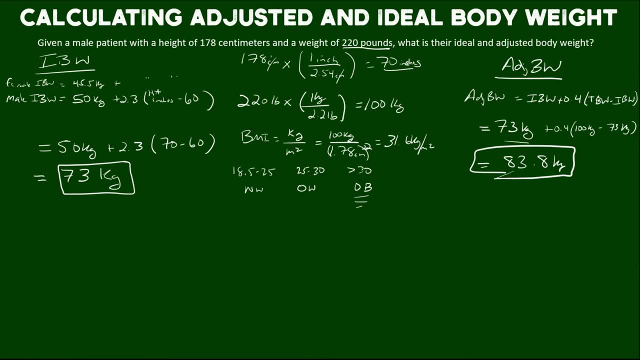 call for ideal body weight. Some call for adjusted body weight. It depends on the patient's body weight. So we're going to go over some of these calculations. Some calculations call for ideal body weight. It depends on the dosing scenario, It depends on the clinical practice site, And so it's. 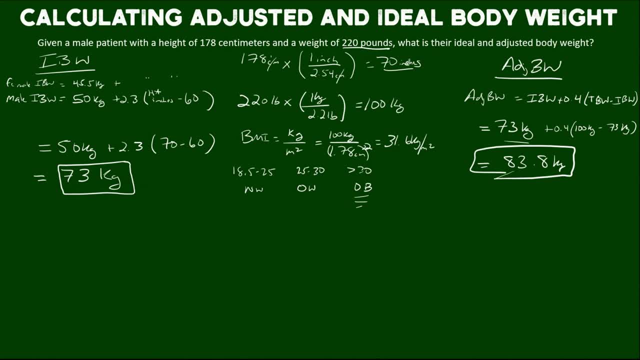 good to know these basic equations so we can quickly do their calculations to get an idea of where a patient's body weight lands relative to what would be the population-based equations that we use. Thank you for your attention. 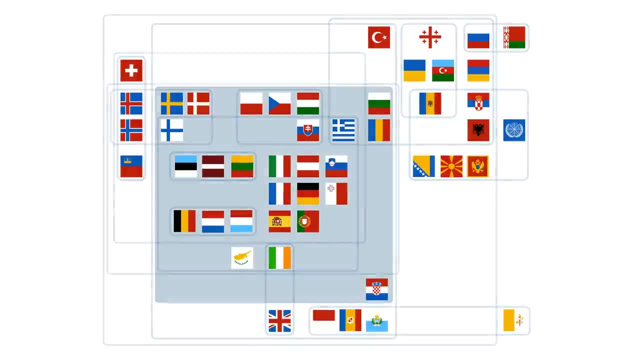 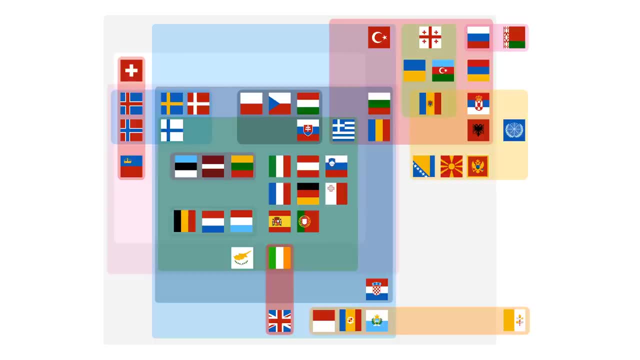 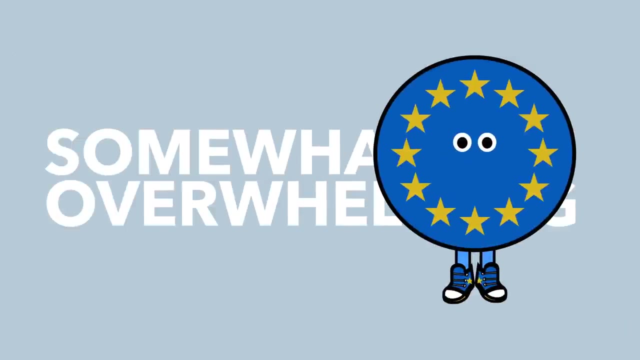 This is the European Union. Well, technically it's just this bit, but all of these parts make up the European Union's network, if you will, Europe's circle of friends. The diagram is somewhat overwhelming, which is pretty appropriate considering. well, that's how many people feel.